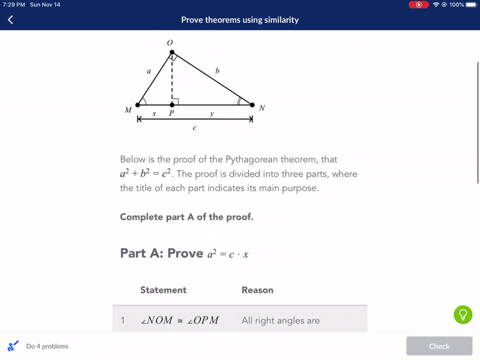 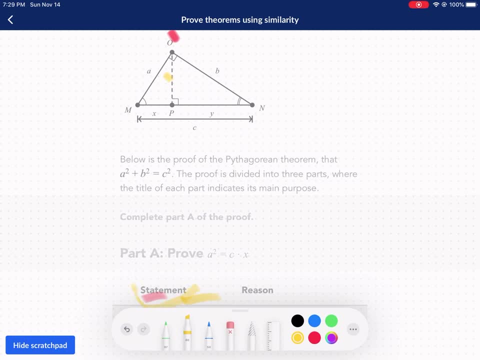 O-M-N. That's a different one. O-M-N. Let me highlight this: This is going to get messy. This is not very conducive to video. However, we'll make it work. Okay, So now we have this angle: O-M-N. That's that green, with that one single line and saying that it's congruent to 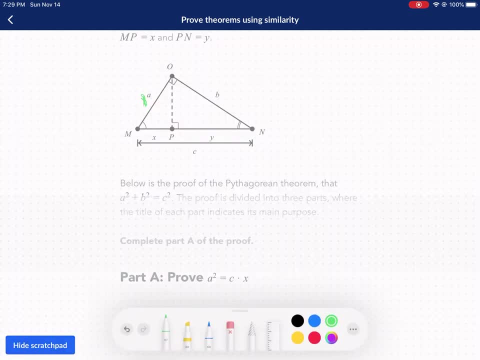 PMO, So I need to find PMO. It just shifts every time: PMO, PMO, Okay. So it's just saying: O Oh shoot, I lost track of that, Okay. So it's just saying: O Oh shoot, I lost track of that, Okay. 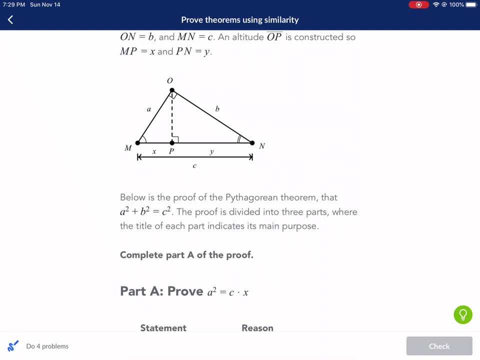 Okay, So it's just saying: O Oh, shoot, I lost track of that. Okay, So it's just saying O Oh man, So O-M-N. Okay, So, look, it's O-M-N and P-M-O, It's the same angle. This is going to be. 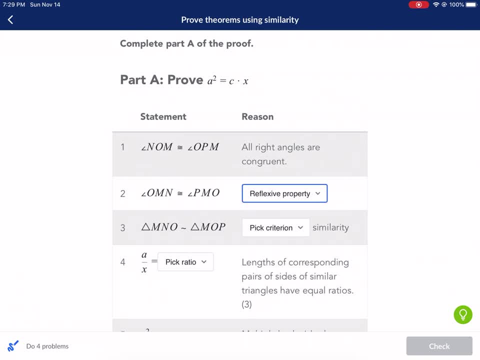 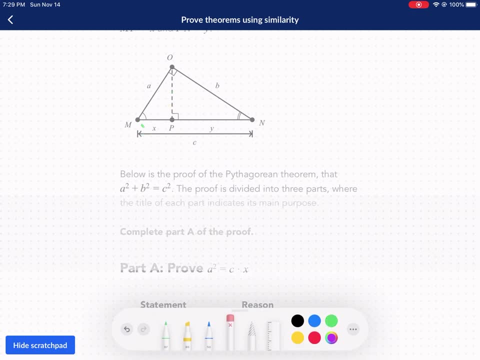 reflexive property. So we're looking for a reason This is going to be reflexive property. What is the reflexive property? Reflexive property is it's the same measurement because it's the same angle. Okay, So what it's essentially meaning is this angle right here belongs to this small triangle. 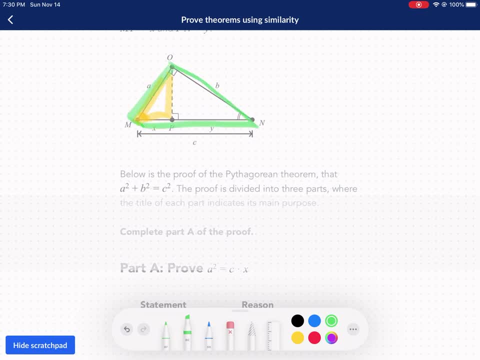 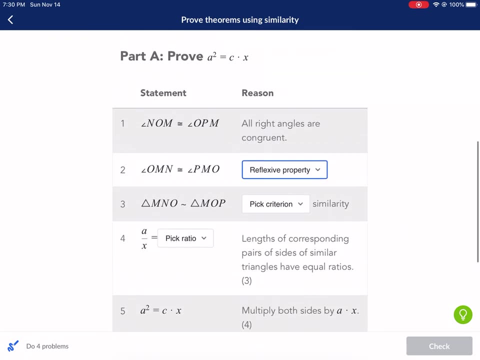 and, at the same time, it belongs to this big triangle and it's the same angle. Therefore, it's reflexive property. Okay, So that's why that's the first one. Okay, Now we're rolling. M-N-O is similar to M-O-P, So now we're going to have Okay, M-N-O. I think that's the. 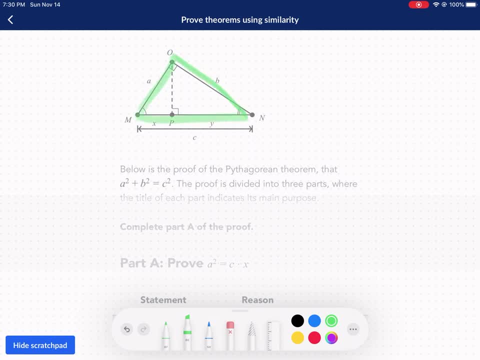 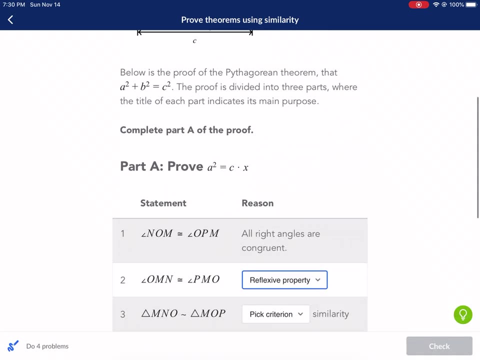 two big ones we were just discussing, So M-N-O and O-M-P, So we're talking about the big one and the small triangle. Okay, There's a small triangle and a big triangle. There's also a medium triangle in there, but it's saying that these are similar because of angle-angle. Okay, 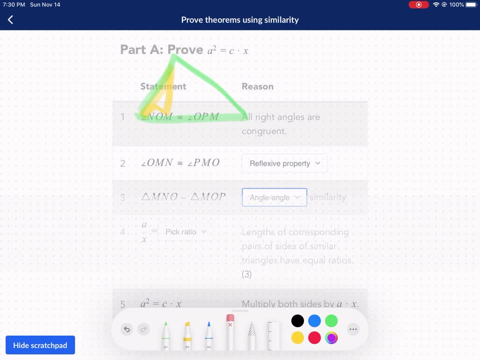 We have two angles here, and usually what you do is if you're, If you Anytime. This is why I always instruct my geometry students. Anytime you're listed a congruent symbol anywhere, you should write a letter, either A or S. In this case it's an. 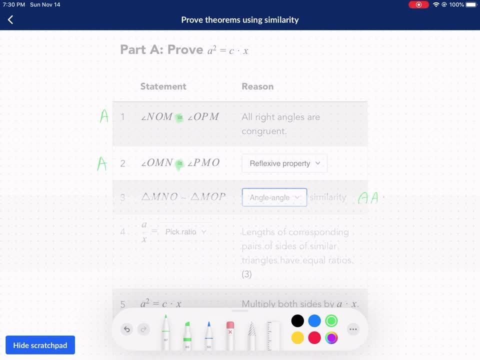 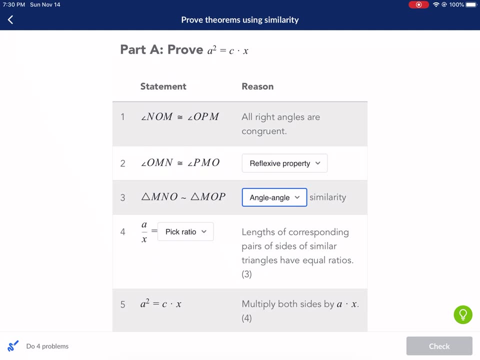 angle and this angle, So naturally this one is going to be angle-angle similarity because of what we've already established here. Okay, So now we have: A over X is equal to some ratio, So lengths of corresponding pairs of sides of similar triangles have equal ratios, Lengths of corresponding. 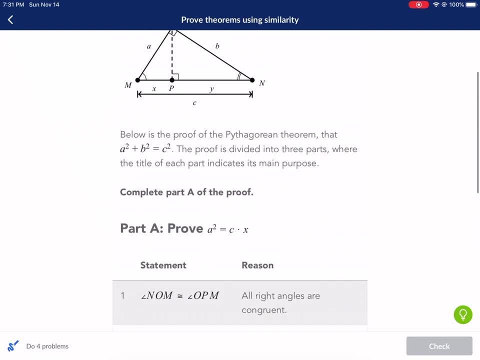 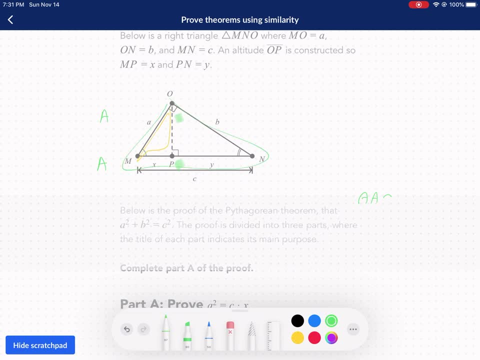 pairs of sides of similar triangles have equal ratios. That's another way to say: if we know these two triangles are similar, Okay, So this yellow one and this green one, if we know they're similar, then we know that, for example, the hypotenuse, 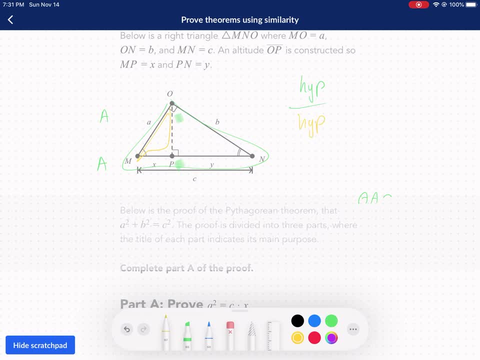 over this hypotenuse over the yellow hypotenuse is going to be equal to the small leg over the small leg. Okay, It's going to have the same ratio. So what ratio we need to find? A over X. So A over X. let's identify the parts. it is for each triangle. So here we have. 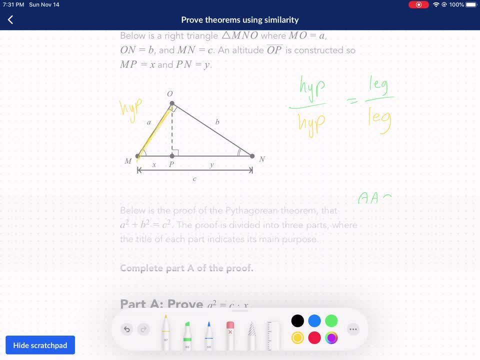 A is the hypotenuse for the yellow and X is this little. we'll call that the short leg. Okay, Now of the big triangle. what does it represent? I should use a different color other than this green. Of the big triangle, what does it represent? Okay, So I'm going to call this. 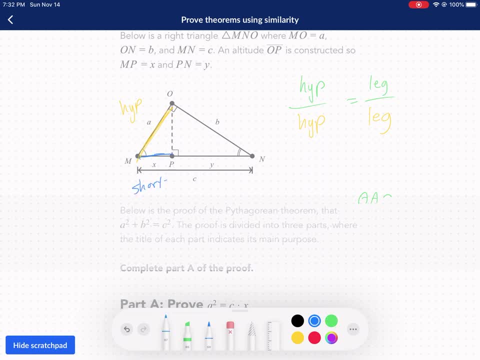 the short side. Okay, So now we have the big triangle. What sides are we representing here in this big triangle? Well, letter A now is the short side of the big triangle, And then this blue X. well, that's not anything, Okay. 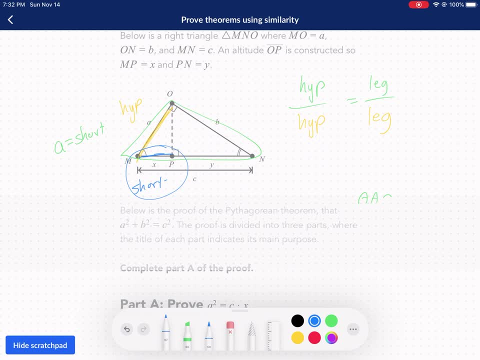 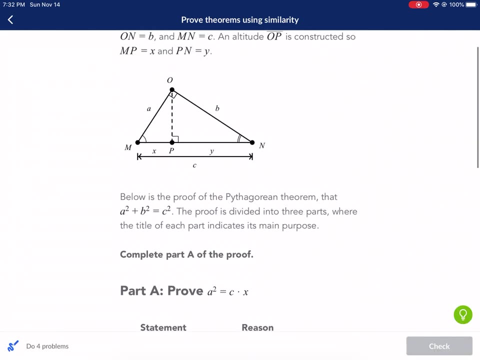 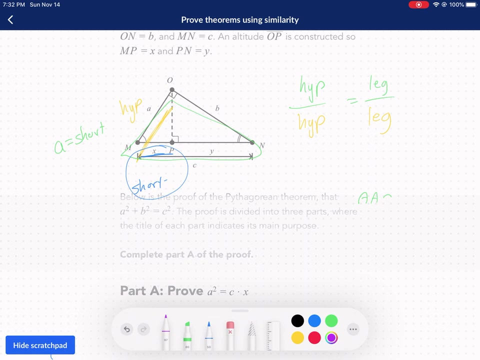 That will. that's not either the short side. It doesn't really belong, Okay. But luckily it's not asking that, It's asking A over X. So A over X is again we're going to say for the small triangle. let me write this out: We're kind of running low on space here. I'm. 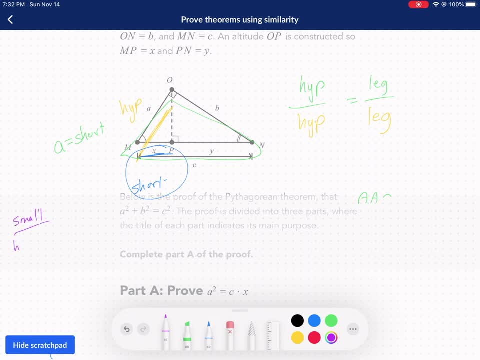 going to switch to all purple. So for the small triangle, we were comparing the hypotenuse to the short side, Okay, And we said that's equal to A over X. Now for the big triangle, we're going to do the same thing. What's the hypotenuse? Remember? we wrote we're comparing. 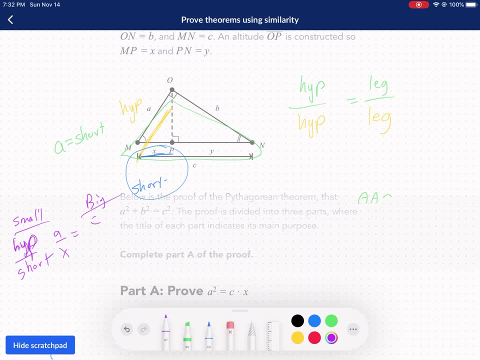 hypotenuse to short side. So what's the hypotenuse of the big guy? That's C. The hypotenuse is C And the short side what is that? The short side is A. That's where we get this, Okay. So it's. 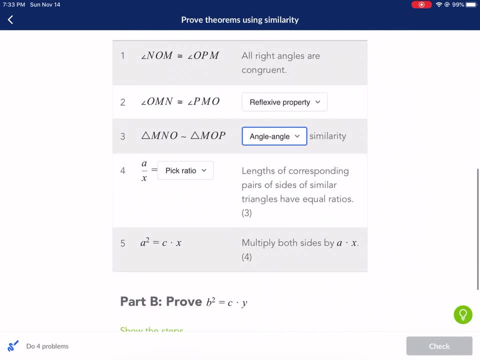 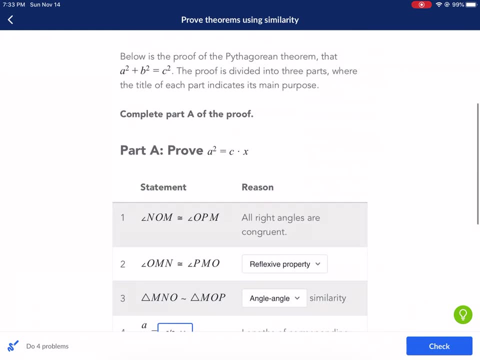 going to be C over A, because that is what it's equivalent to. So let's go C over A, that one, Okay. And then we have multiply both sides by X and we get that formula. A squared equals C times X, I think. 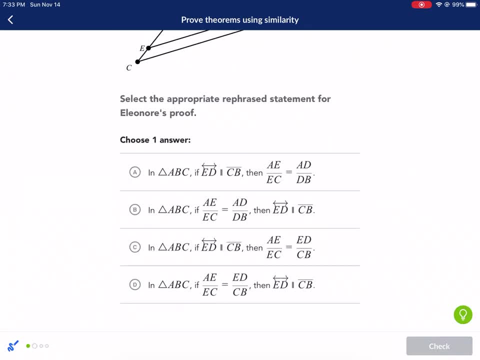 we're supposed to check it right. here We are. Okay, I think it's going to go on to part B. No, it's not. We don't even go to part B. That's disappointing. Okay, Here we go. New one: 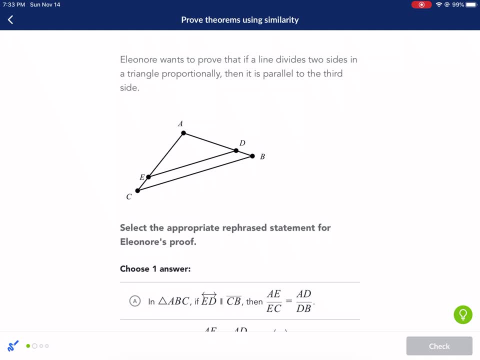 Eleanor wants to prove that if a line divides two sides in a triangle, proportionally, then it's parallel to the third side. Select the appropriate rephrase statement for Eleanor's proof: Oh boy, Okay. So here we go. Eleanor wants Eleanor. Eleanor wants to prove. 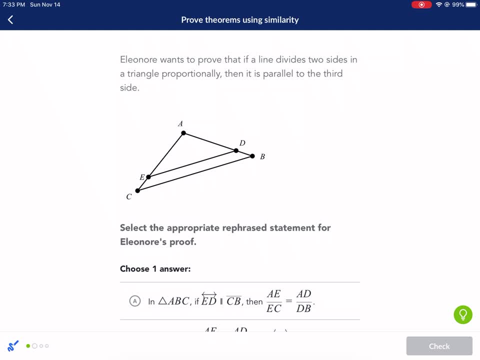 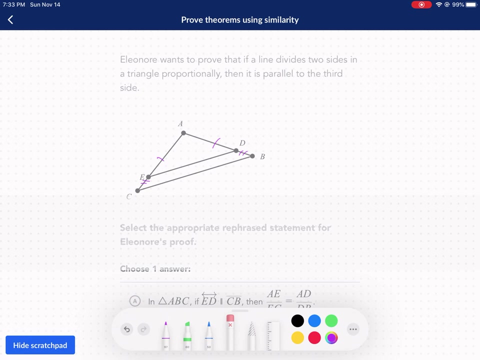 that if a line divides two sides in a triangle proportionally, then it's parallel to the third side. Okay, This is one of those kind of it's kind of those obscure theorems. It's saying: if it divides this proportionally, So that okay, If it's something like that, where C, E, whoops. 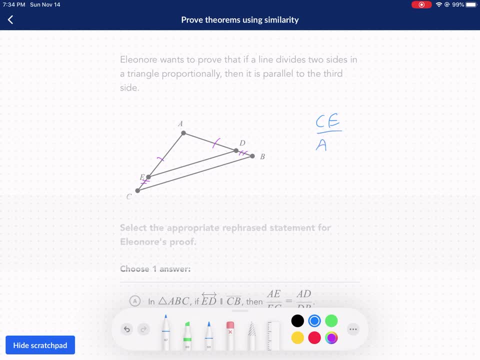 I thought it was writing C E over A E. we'll call that. Oh, actually, no, that's not the side of the triangle, So just rewind here. I'm trying to highlight. All right, here we go. So we have this, we have a big triangle here. First, 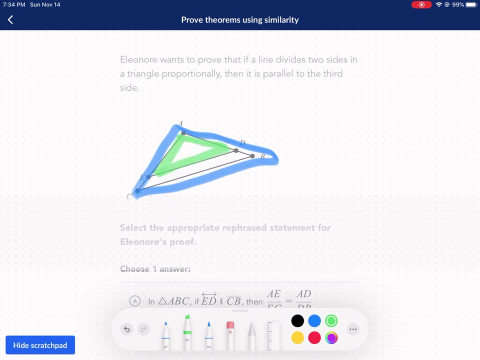 let's identify our triangle. So we have a big triangle here, Then we have this green triangle. Okay, Now we're rolling. If we have A E, which is that small side, over A C, Okay, If that is proportionate meaning to this other side, So we could say, uh, divides two sides into. 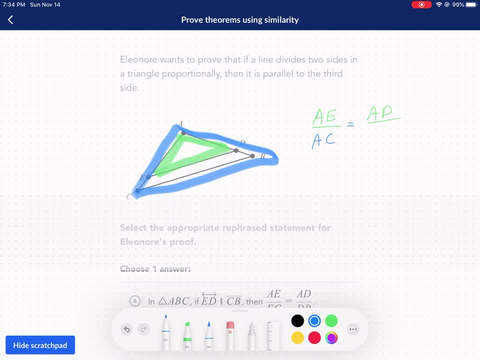 uh, triangle proportionality. So A D over A B. Okay, Those are the sides. So A B is that big side And then A D is this side. right here, Basically, I'm saying the sides of these triangles compared to each other, the small to the big. Okay, So the small obviously is on top and I put 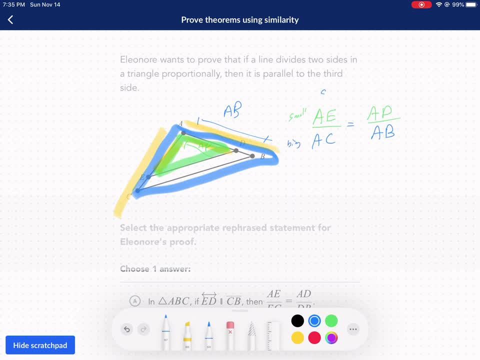 big on the bottom and I have the different sides Okay, So this is like left side and this is right side, Right, Okay. So I'm just comparing the different sides. If that is proportionate, then we know that this is parallel, right here, Those two lines, Okay, And that is. that is the. 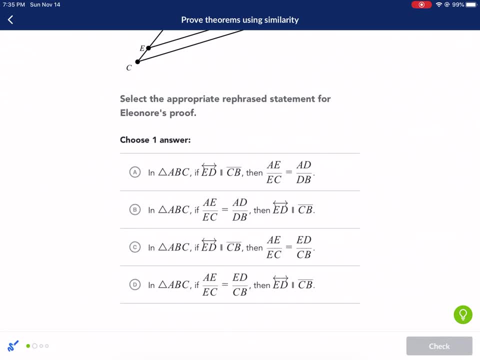 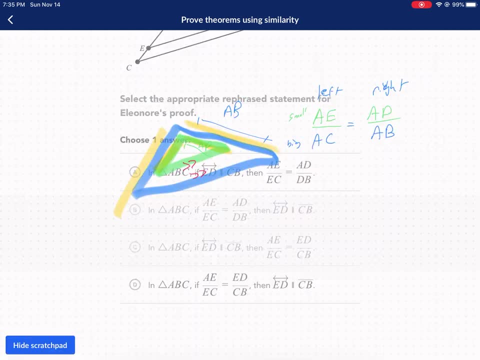 theorem. So we need to see, okay, If in ABC, if E, D is parallel to CB, no, it's not saying if it's parallel, it's saying it's proportionate, then it's parallel. Okay. So because the the parallel. 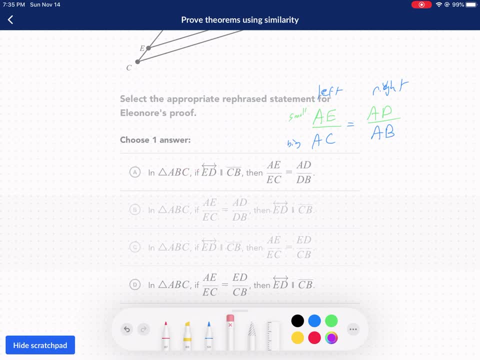 statement is second. Okay, I'm going to leave that up there, because the parallel statement is segment second. Then we know that we're either looking at this guy or this guy. Okay, So C and A are parallel, because we're proving that the lines of parallel based on the proportionality. Now we just 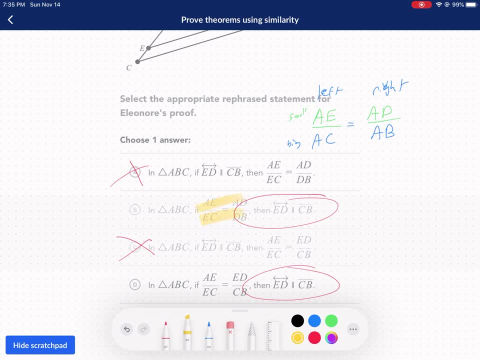 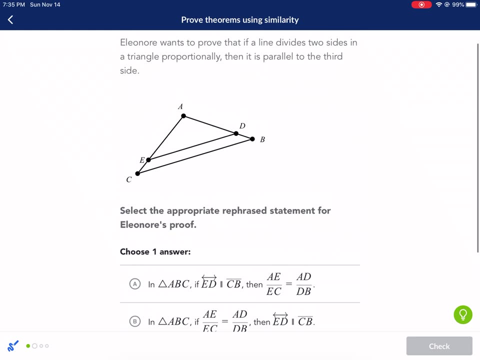 need to look here and see which proportion is correct. Is it AE over EC? Okay, Let me go up and look real quick. AE over AC, no EC, Okay. So that's fine too. You can also do it that way. 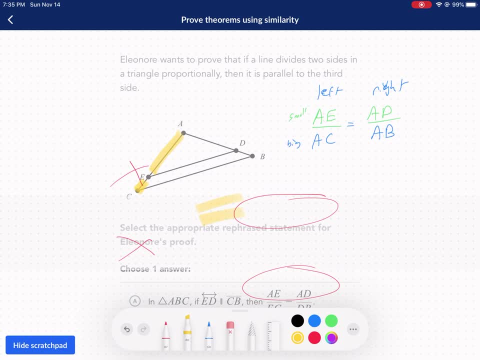 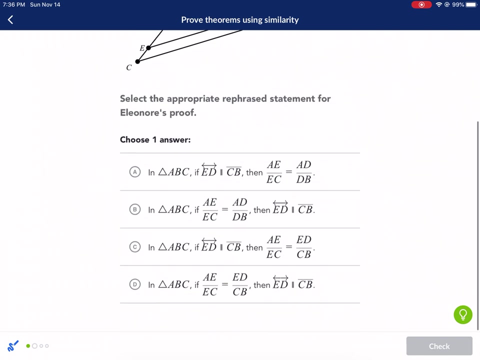 So AE over CE, that little. so the kind of the top segment versus the bottom. So you can do a top to bottom Okay, But it also needs to be equal to the top of bottom on the right side. So that's gotta be AD over DB. So we need to see which one says AD over DB And that is. 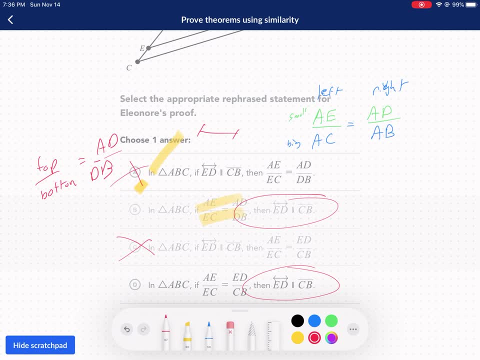 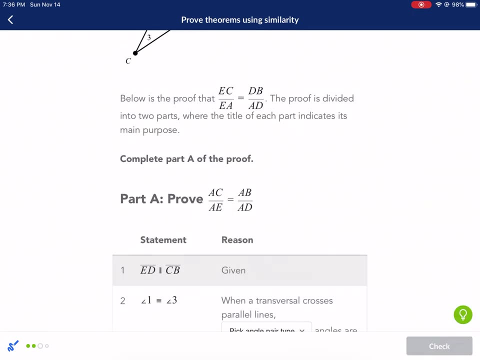 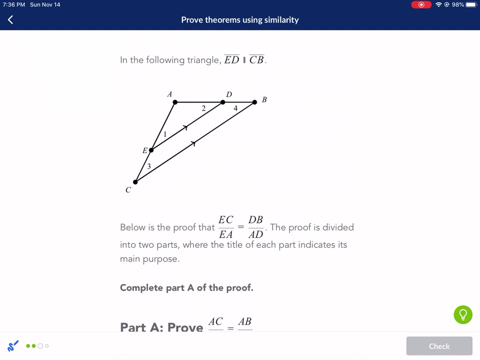 letter B. The other one says ED and CB. That's not correct. We have to do the same proportion we had in the other one. So it's option B. We're going to check it. Next question: Okay, And the following: ED is parallel to CB. Okay, So now it tells us that it's parallel. We're 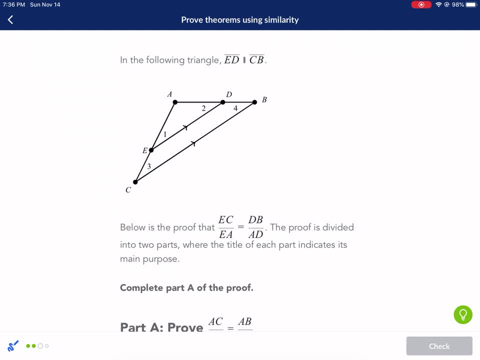 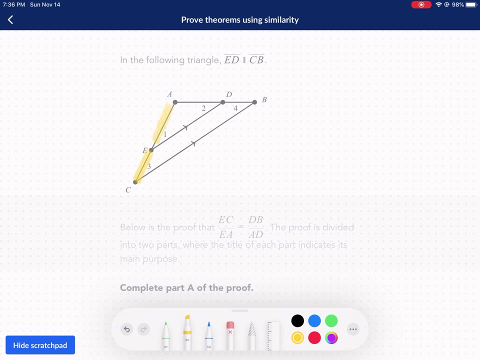 going to reverse in the exact opposite, or exact opposite direction than the previous problem. Below is a proof That: EC over AEA. there's a lot of looking at different lines here. This is super geometry, but that's okay. So EC is where, EC over EA, Okay. So again we're doing top to bottom. 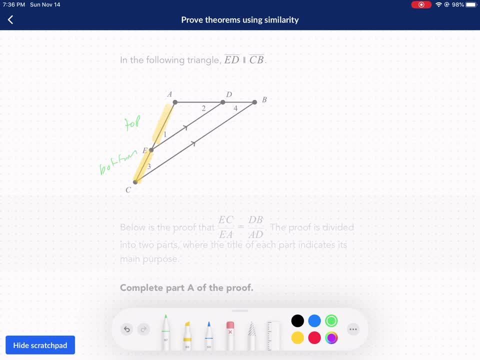 which you can do: top to bottom, proportionality and DB over AD. Okay, So top to bottom, on the right side too. So top, well, actually it's putting the bottom on top, which is fine, but I hope you guys know what. that's what I meant. 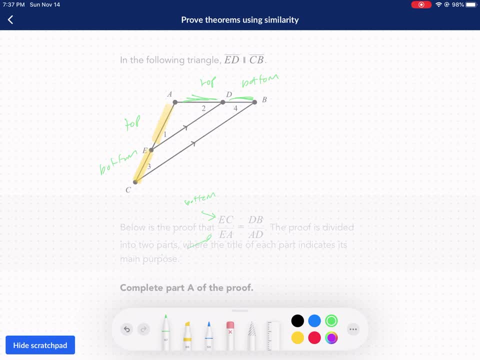 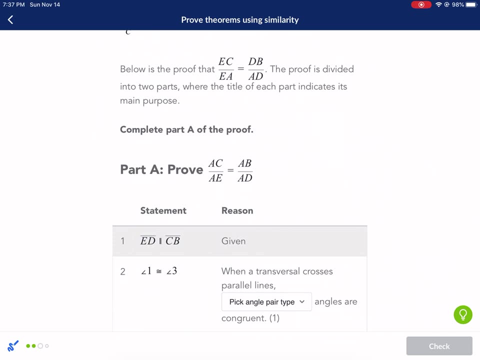 That's the bottom side or the bottom portion, And that's the top portion. Okay, So now let's go back over here. The proof is divided in two parts where the title of each part indicates its main purpose. Complete part A. So we're only interested in part A, AC over the thing we had just looked. 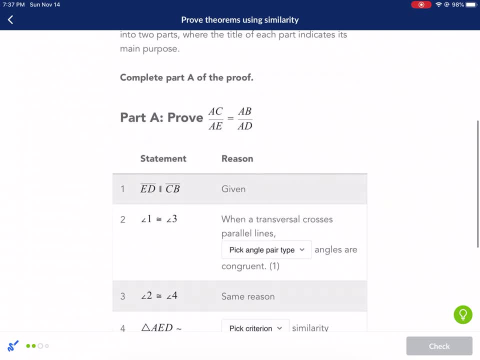 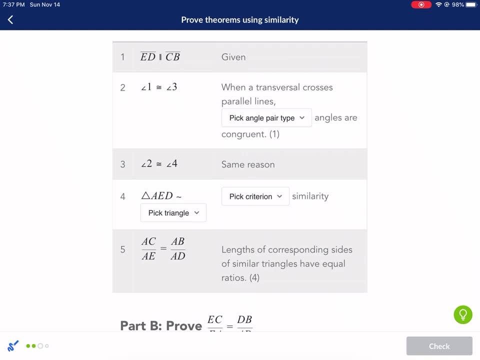 at. So ED is parallel to CB given. Okay, That's our given. Now we have a congruent sign, So we're going to either put like an angle here or something. When a transversal crosses parallel lines, blank angles are congruent. 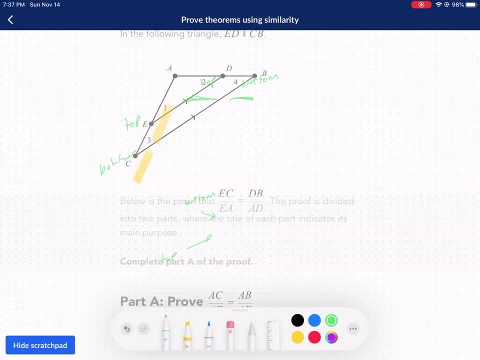 Okay, So when a transfer? so we're looking at one and three here- let me erase some stuff- We're looking at one and three. I already know what this is, but I want to highlight to you guys. So here we have these two lines parallel and then one and three are created because we have 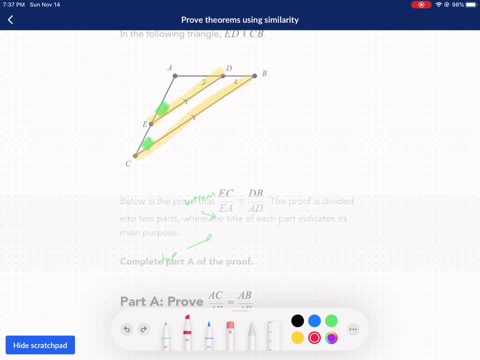 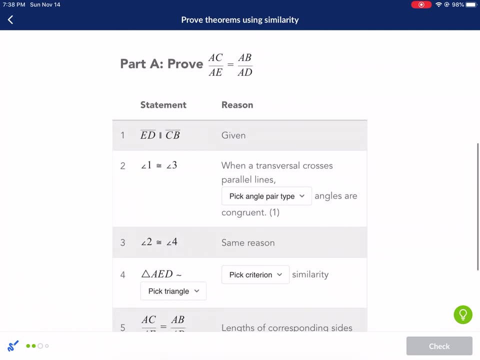 this transversal here and I'm going to make it in red: this transversal. Those are corresponding angles. They're in the same part of the intersection. I like to say, if you want a brief of that, I have plenty of videos on that, but these are corresponding angles, Okay. 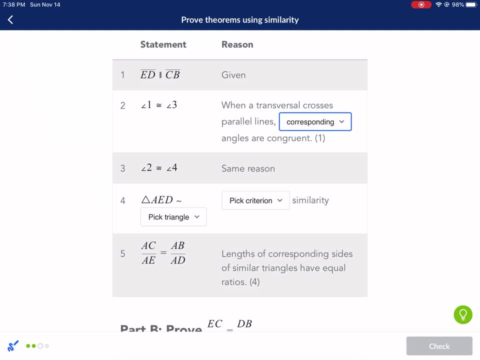 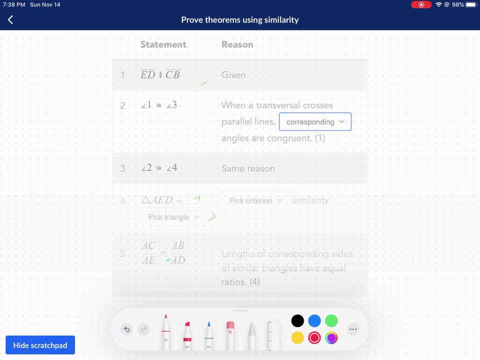 Now angle two and angle four. the same reason: corresponding Note that we have. we'll get rid of that Note that we have two angles that we're proving here, So I'm going to put A and A. Now we have. AED is similar to something. Okay And based on what type of 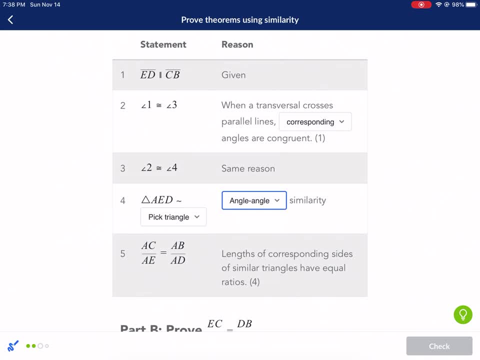 well, it's going to be angle angle, because that's all we have. We have angle, angle and that's it. But what type of similarity? is it going to be AED? Well, we need to identify where AD is AED. 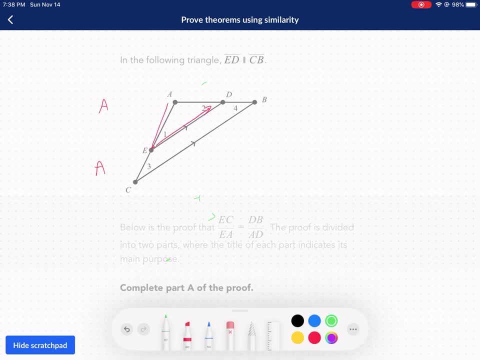 AED is going in that direction And we need to duplicate that direction for the big triangle. So ACB, triangle, ACB is the big one. We have to do it in the same order And then that's going to be congruent. no similar- sorry, similar- to triangle AED. If you wrote ABC, that's a different. 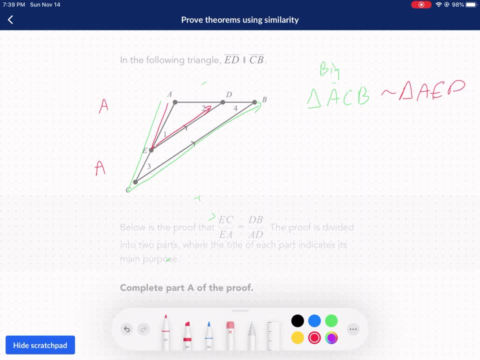 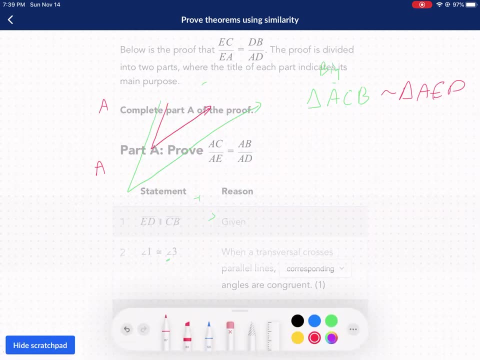 triangle. It has to go in the same order because those angles are in reference to each other. Those angles need to be the same. So angle A needs to be the same As what did I say for that one: AED, ACB. So ACB is what I'm looking for, ACB, Because A needs to. 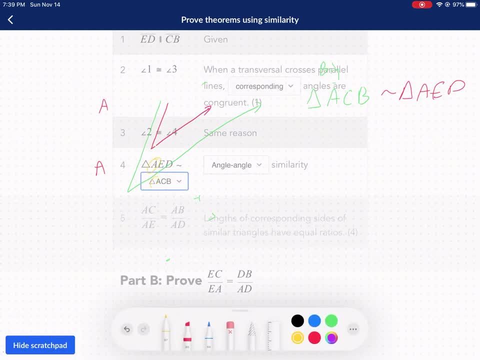 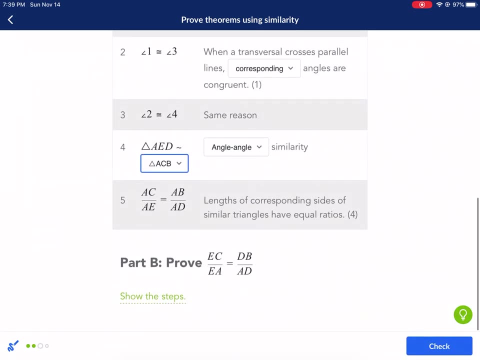 be congruent to A, A needs to be congruent to A, E needs to be congruent to C And B needs to be congruent to D, in that order, Okay. So that's why that's the way it is, And I think that's all it's. 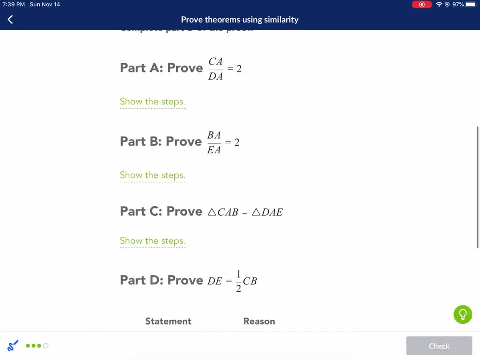 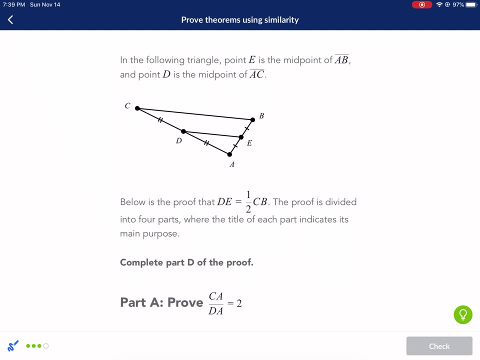 asking Part A. check it Next question. Last one, Actually not too bad, Oh my gosh. In the following triangle, point E is the midpoint of AB And point D is the midpoint of AC. Just a critique for maybe Khan Academy creators. It's a little. 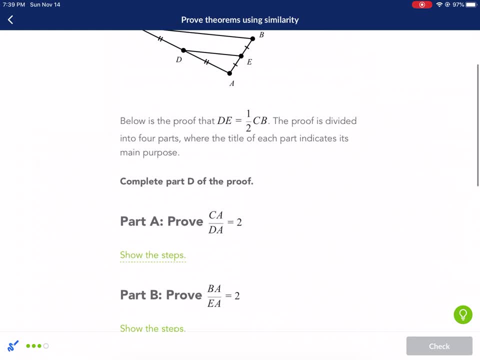 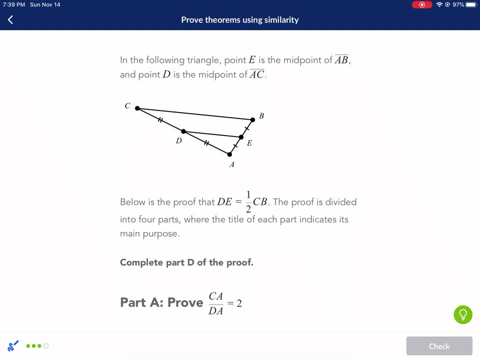 confusing just because we're jumping around all over the place. I get what you guys are trying to do, But maybe just have like break this up into a couple of okay, anyway, they're probably not watching this video anyway. In the following triangle, point E is the midpoint of AB and point 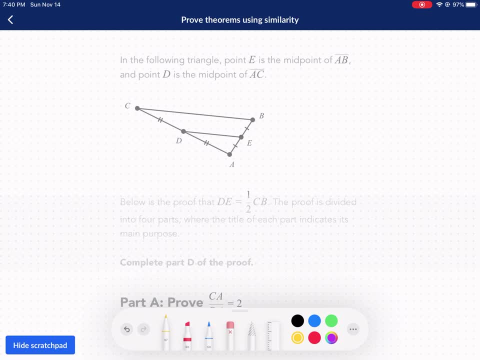 D is the midpoint of AC. Okay, And you can tell that because it's got these lines right there. Okay, Those lines indicate midpoint. So that's the midpoint. That's the midpoint. Below is the proof that DE equals one half of CB. That's another theorem. That's actually a pretty useful one, This green line. 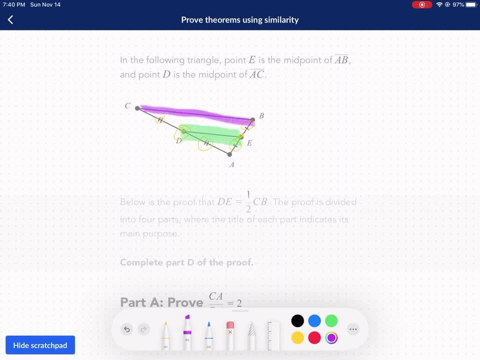 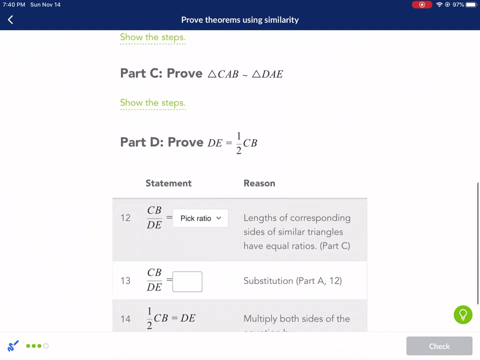 is half of this purple line. Okay, So that green is half the length, which is kind of cool. So you multiply CB times one half in order to get DE. Sometimes that's a little confusing for people. The proof is divided into four parts. We only want to worry about part D. Okay, So CB over. 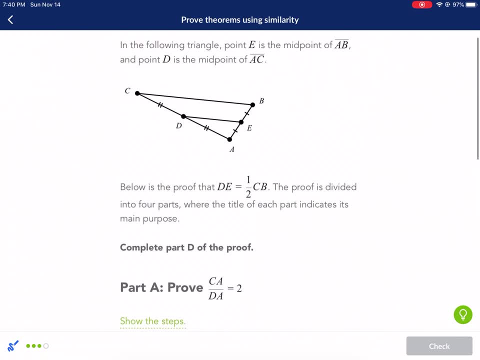 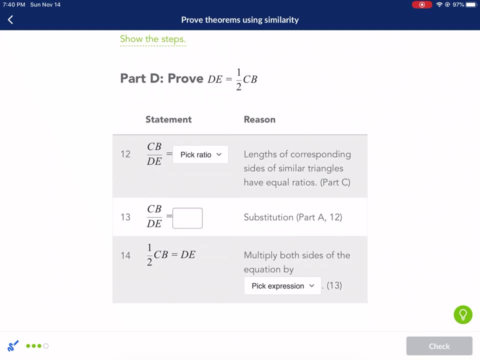 D to E equals blank. Okay, So we knew that CB is the long side and DE, So we know that's two to one. right, But it's looking for proportion. So CB over D to E is equal to what are our options? 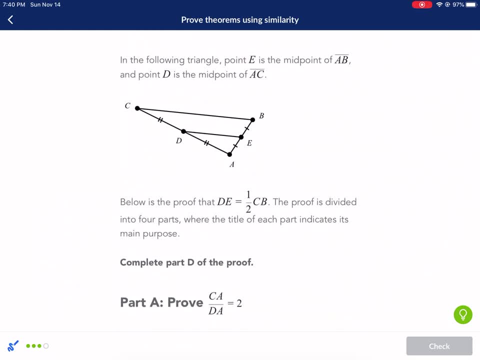 Boy, I wish I let me jot down. So we have CB, So one of our triangles is this. I'm just going to write it down because I don't want to go back and forth. So we have, this is the big triangle. 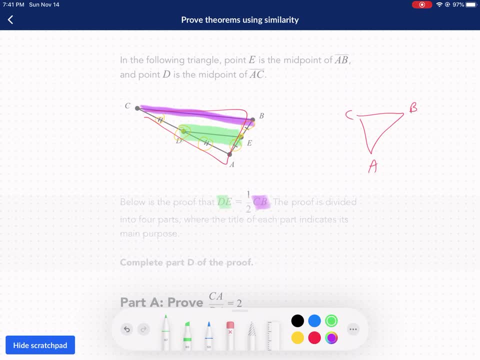 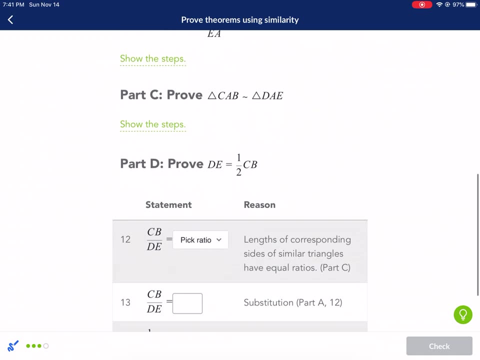 We have A, B, C- I swear I'm not this bad at drawing- And then we have A, E, D. Okay, In that order. make sure that you keep that order the same. So I'm going to scroll down here and now I can look at it easier. I'm going. 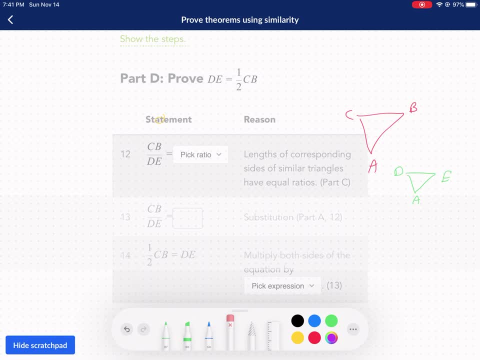 to erase this. Okay. So then it says CB, that's this line, over DE, That's the bottom side, is going to be proportionate to what? What are our choices? We have CD over DA, CD over DA, CD. Okay. 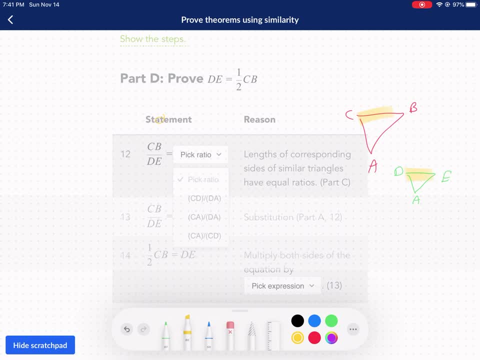 Portion. then DA is CD, CB over DE. We're looking at the whole side. So that's not going to work. Okay, We want like CA over AB. So we have CA over DA, CA over DA. That's going to be the one, Okay. 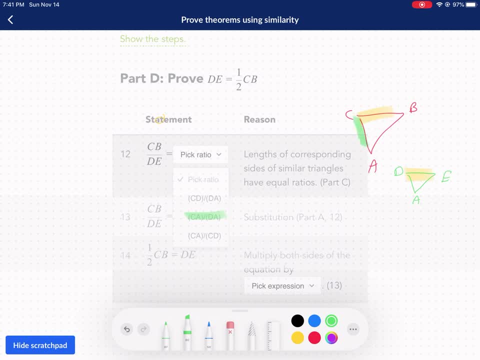 So our second one is it: How do I know, Because it's this whole length of the side there And this whole length of the side there, Notice how I don't see CD in this triangle. So I know the top one's out, CA over CD. 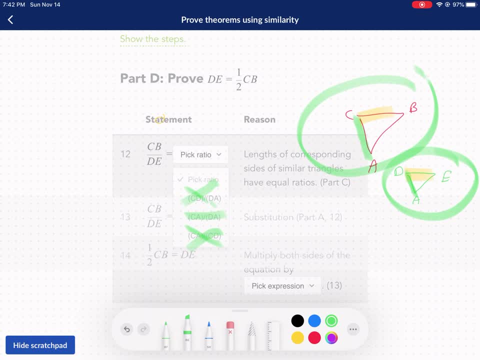 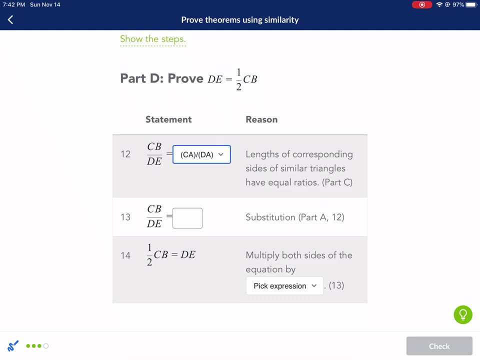 There's no C in this second triangle, So this option's out. So it's CA over DA, CA over DA. Then we have CB over DE is equal to substitution. So we're going to substitute part A12.. Well, I don't even have part A in there, Let's see. Hold on, Maybe I got to look. 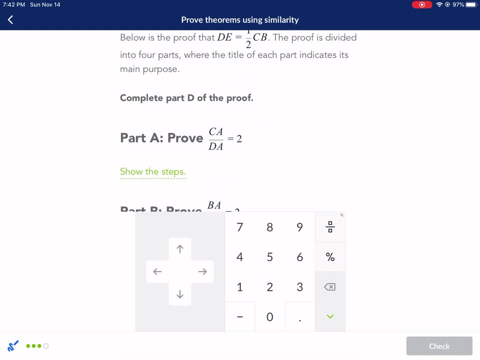 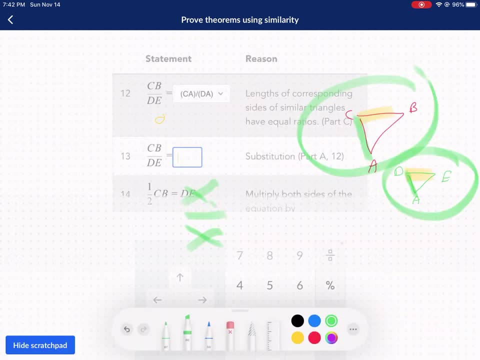 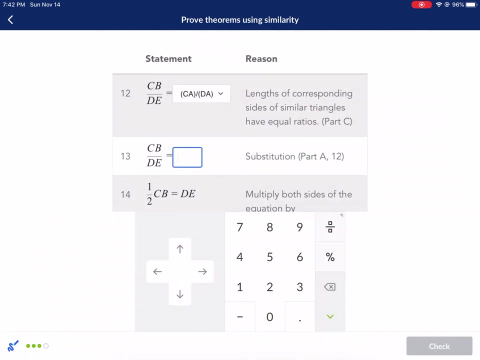 I got to show this up: CA over DA equals two. So hold on. I got to scroll down here: CA over DA equals two. So I looked up at my part A and it said- let me erase this. It said that this CA over DA is equal to two. So I'm just going to put: this is equal to two. 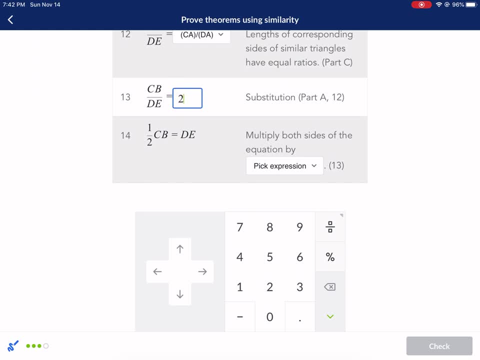 if I'm using substitution And then one half CB equals DE, Multiply both sides of the equation by how do I do this? So I would multiply both sides by DE, Probably one half. I need to get to one half And I multiply. I think that's going to do it. So how does this work? Okay, If you have. 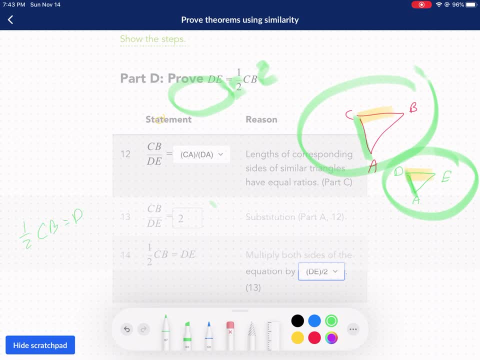 one half. you're going to multiply both sides of the equation by. how do I do this? So I would multiply one half: CB equals DE- Oh sorry, I had this, I started here. CB over DE equals two, And if I 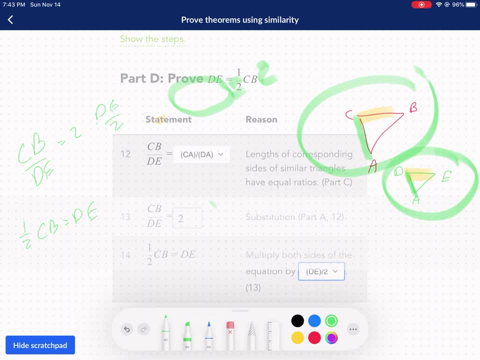 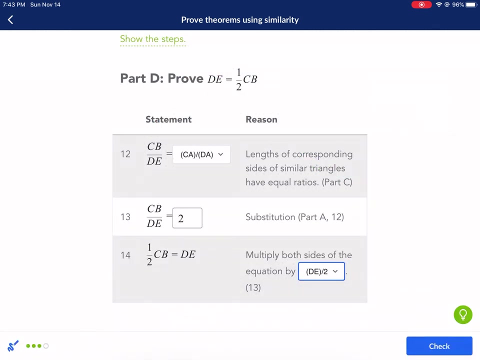 multiply by DE over two. I have to multiply that to both sides. Sorry about that, Okay, And what happens is this cancels out, these cancel out, and I'm left with CB over two equals DE, which is the same thing as one. half that, Okay. So D over two, And there we go Finally. 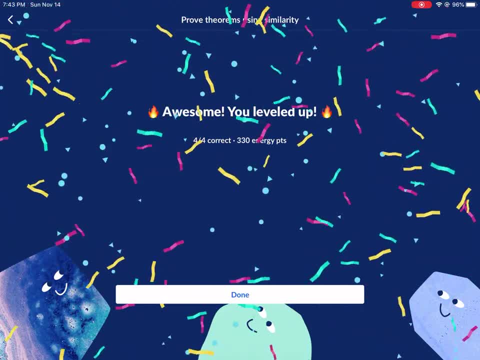 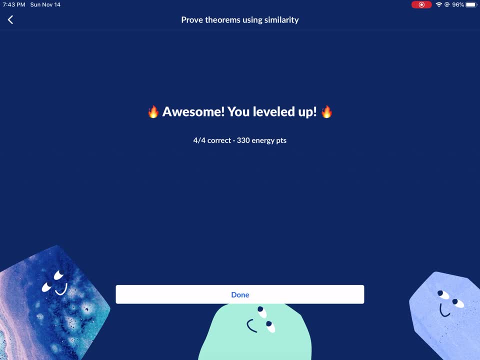 that's it. Okay, That's a tough one. Thank you for requesting that video, So I hope that helped a lot of people out there trying to learn about geometry and proofs. It can be very challenging. I have a lot of videos that are non-Con Academy related. If you ever want to search those up, you can type: 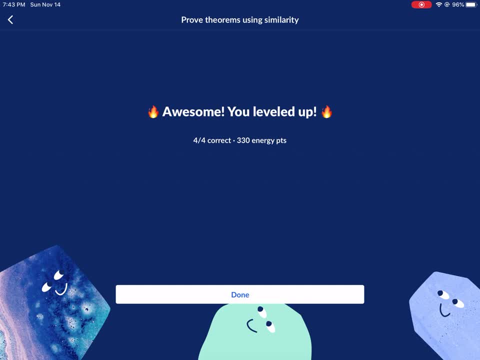 improve or I can't remember. It's been a while since I even had them, but just go look at my geometry notes. I have a lot of note sections in there for the Pearson book And if you need another video, leave a comment. I'll do my best to answer it. Either way, I look forward to seeing you, right.